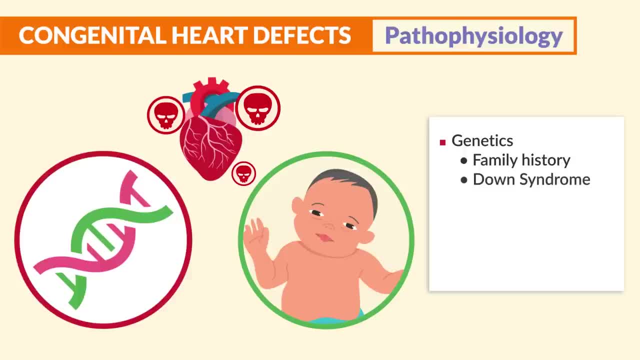 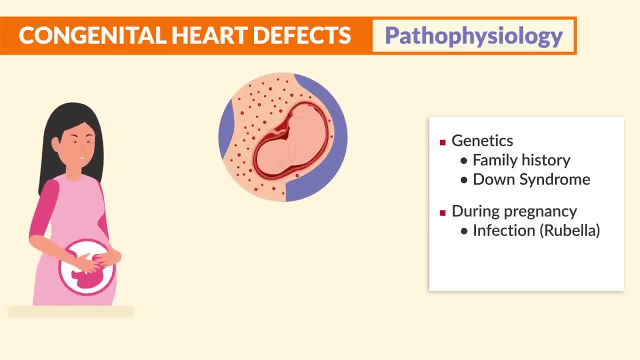 So family history of heart disease and Down syndrome predisposes a child to congenital heart defects, And even during pregnancy if the mother has infection like rubella or uses alcohol or drug abuse and even diabetes. all these things are huge risk factors. 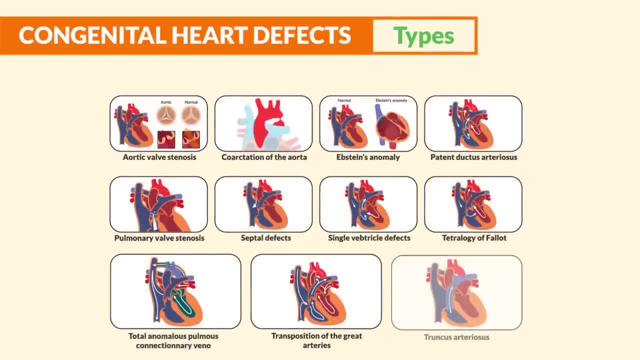 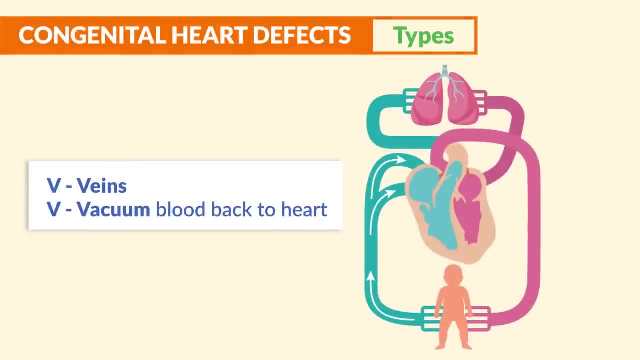 Now, in terms of the types, we're going to break down all the pathophysiology signs and symptoms and treatments for all the top tested cardiac defects. But first let's cover some key points that apply to all of these. As you know, in a normal healthy heart, deoxygenated blood is vacuumed. 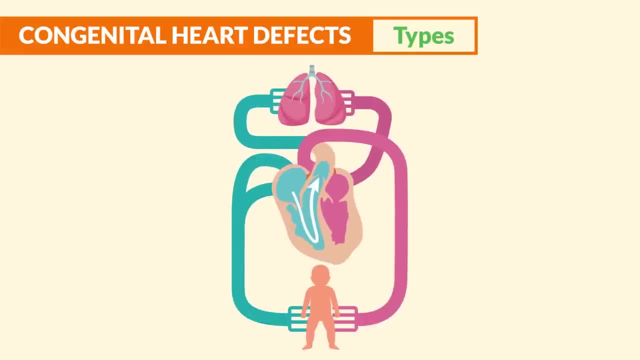 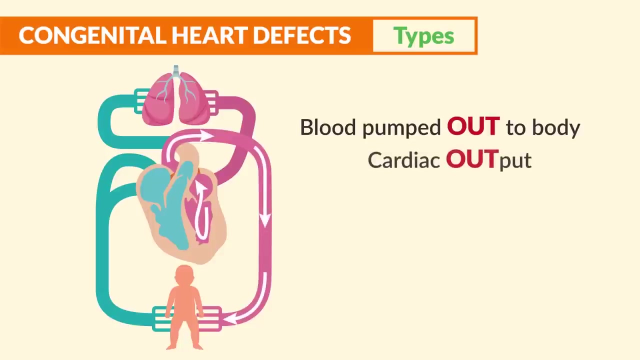 back to the heart via the veins, through the vena cava and into the right side of the heart, Then pushed into the lungs to get oxygenated. After that, this oxygenated blood is pushed to the left side of the heart to be pumped out to the body. This is called cardiac output. 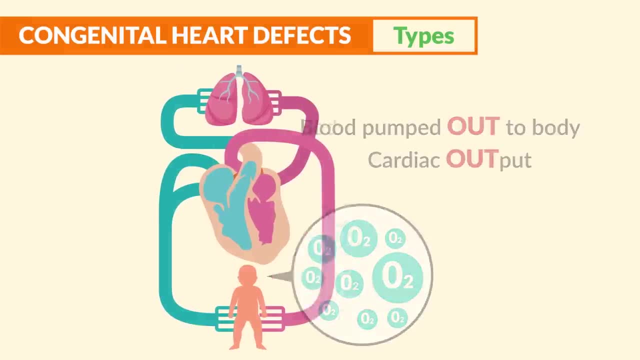 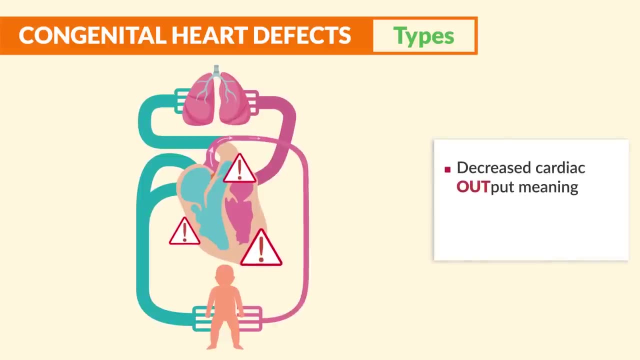 meaning oxygen-rich blood out to the body. But with these heart problems, less blood is pumped out of the heart, resulting in decreased cardiac output. meaning less oxygen-rich blood out to the body In big complications like abnormal heart rhythms, murmurs, heart failure and hypoxia. 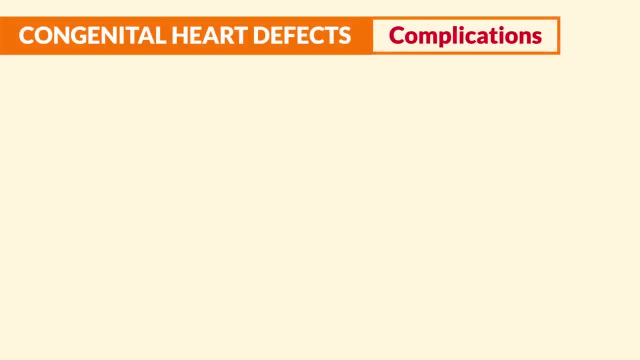 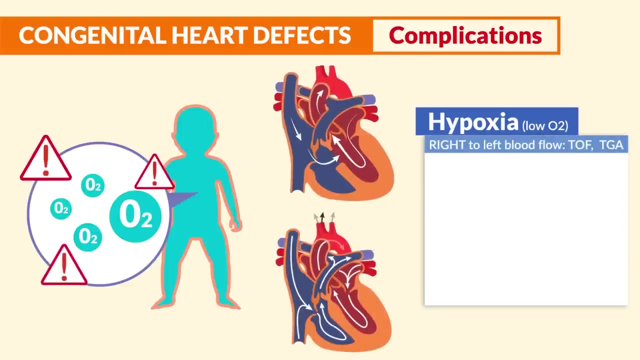 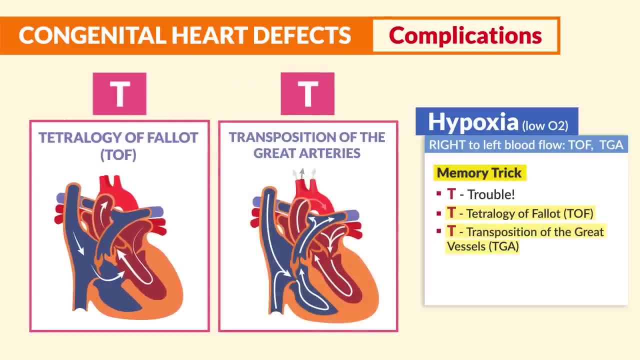 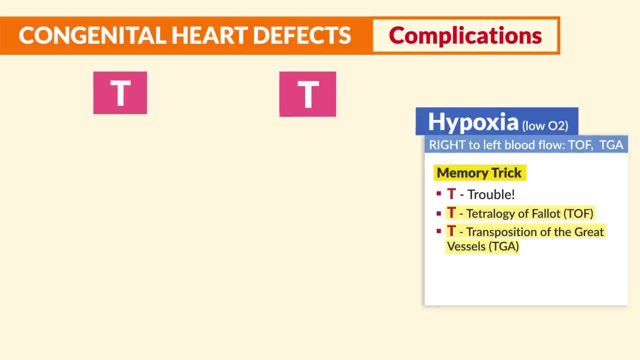 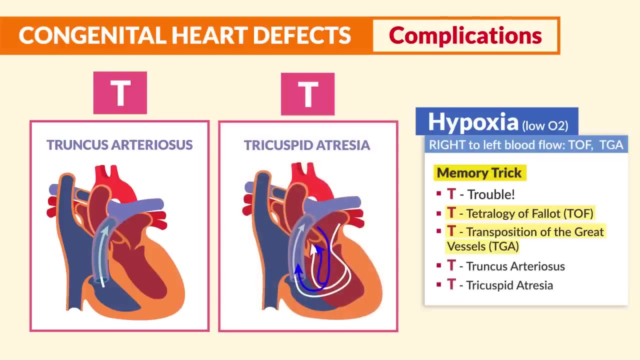 for transposition of the great vessels, TGA. So these are the two most tested, so please be sure to write these down. Now the last two T's: we have truncus arteriosus and also truncus atresia. Now we'll break these down one by one in a moment, but first you must remember that these are: 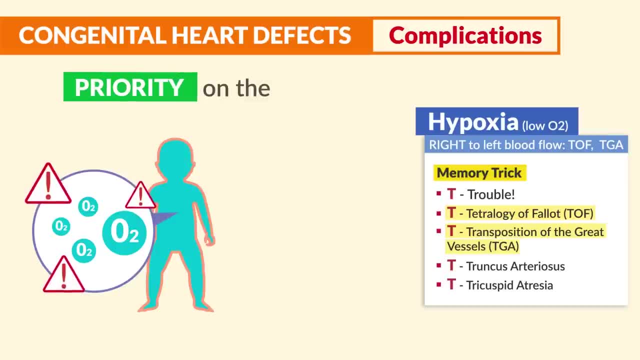 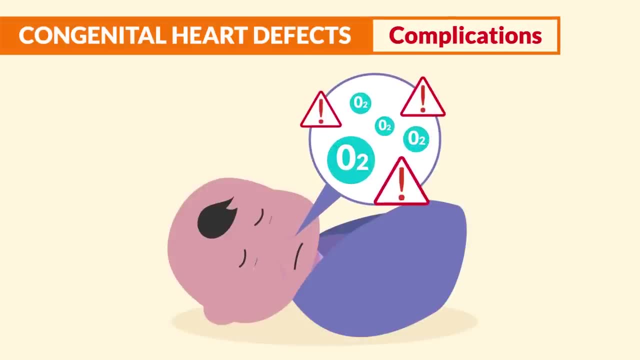 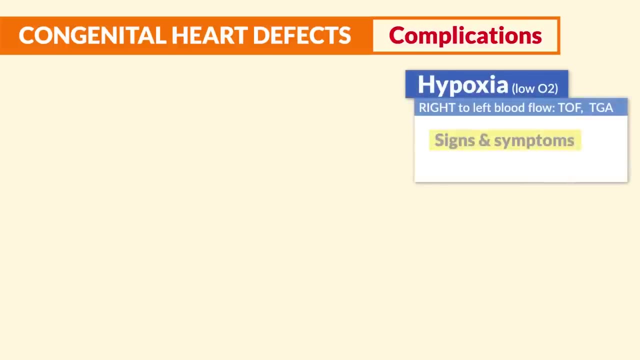 priority, since low oxygen is always a priority on the NCLEX, since it's the most deadly here. Now this hypoxia leads to blue babies, as these defects take blood away from the lungs and push it to the left side of the heart. So top signs and symptoms to write down is number one, cyanosis. 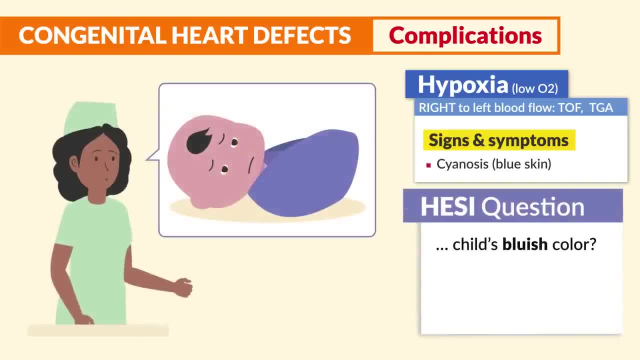 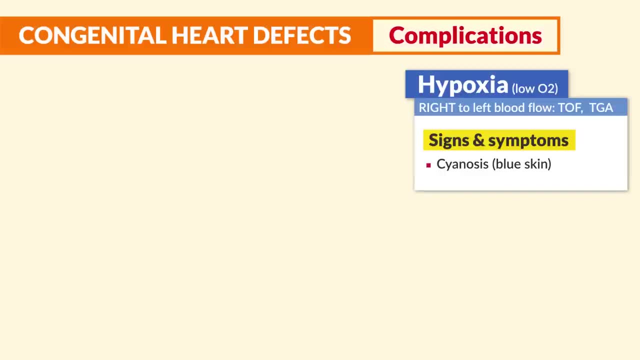 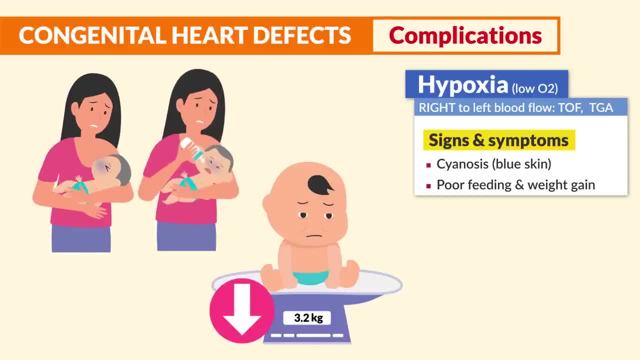 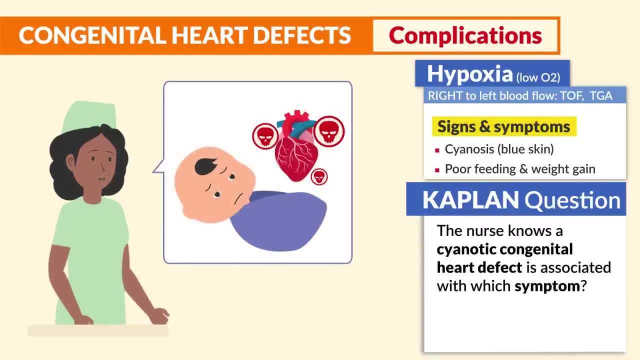 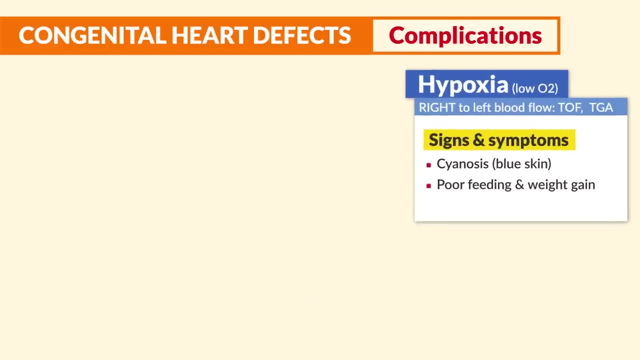 from that lack of oxygen it's harder to breathe during feedings. So Kaplan mentions the nurse knows a cyanotic congenital heart defect is associated, with which symptom: Poor feeding with no or very poor weight gain. The next sign and symptom is clubbing fingers, those thick. 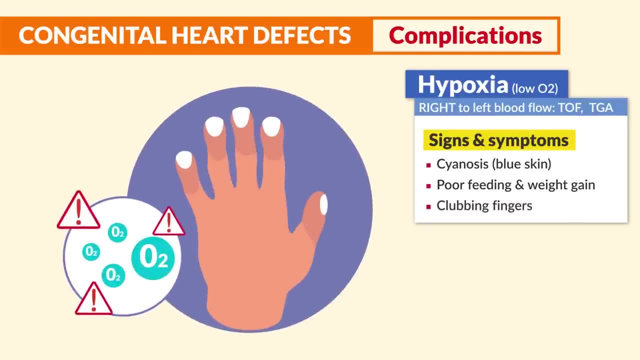 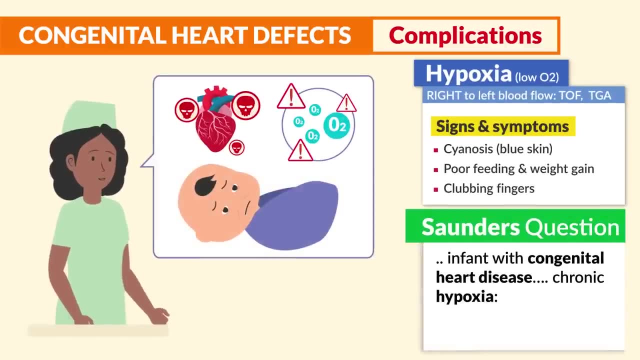 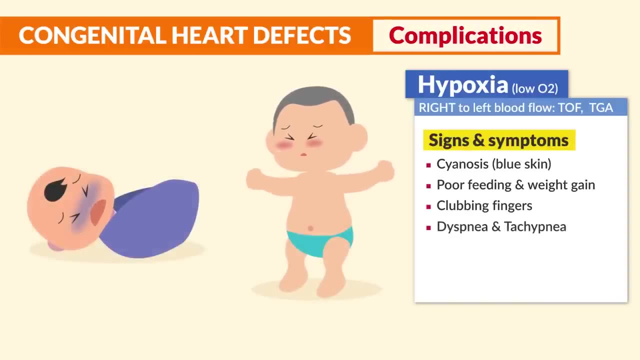 spoon-shaped fingernails from that low oxygen. So Saunders mentions an infant with congenital heart disease, Toxia. We're most likely to see clubbing of the fingers. The next sign is dyspnea, as well as tachypnea, that difficulty breathing and fast respiratory rate. Now a big sign here is. 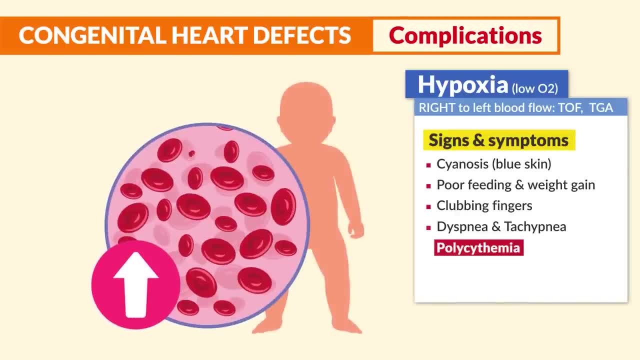 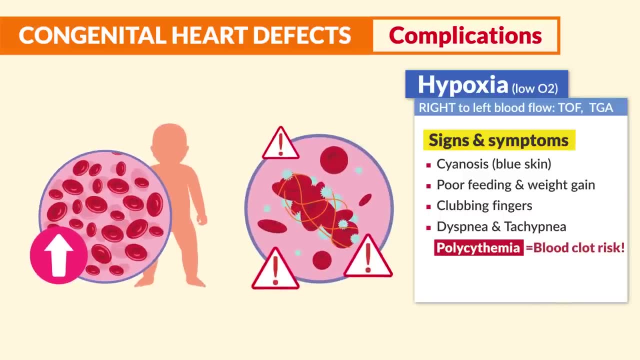 polycythemia. This refers to an increase in number of red blood cells within the body, So huge blood clot risk. So please be sure to write this down. We always report a hemoglobin level over 22.. Huge NCLEX tip. 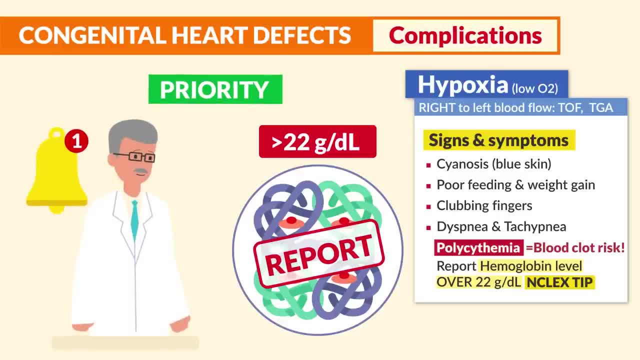 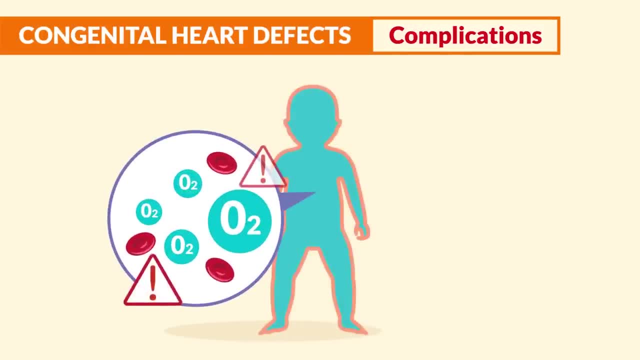 Now, this is priority and must be reported to the health care provider. So please be sure to write it down. Many students get this wrong. Now here's why, Due to the hypoxia in the body, the body says: oh snap, I better make. 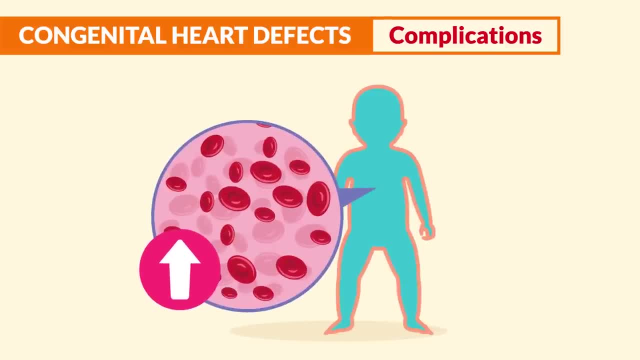 more oxygen carriers. So hemoglobin is produced to compensate for this low oxygen. But instead of perfusing the body, these extra RBCs cause a big old traffic jam within the blood vessels. Basically meaning we must stop my hemoglobin levels, and stop my hemoglobin levels Now plus. they're just the combination. 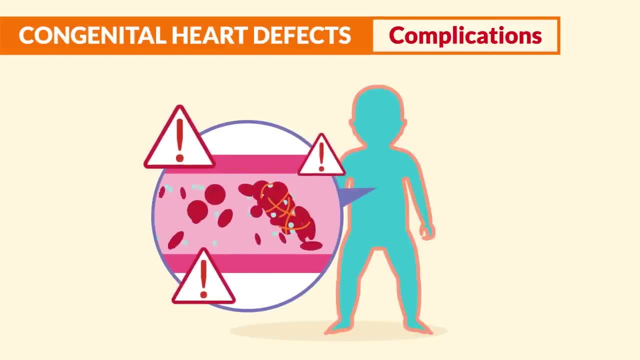 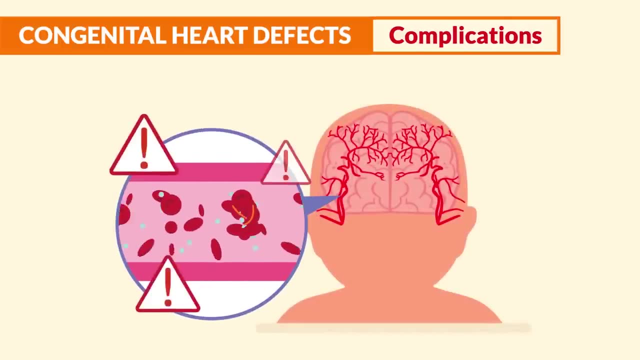 of the blood cells. I mean, if they had to be exactly the same, I'd probably be able to get rid of these things and get rid of them. I do have a legend here, but I'm gonna show it to you. In the blood clot of a human there's thick, viscous blood that can easily clog tiny little blood. 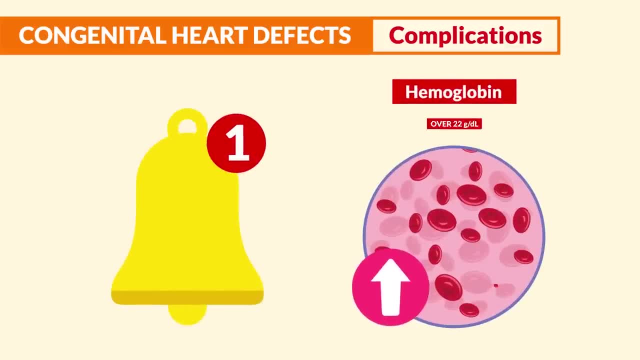 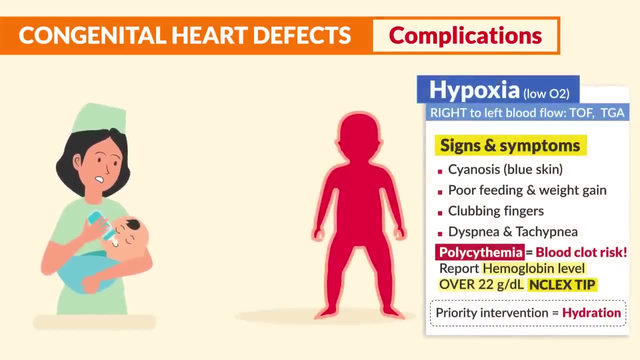 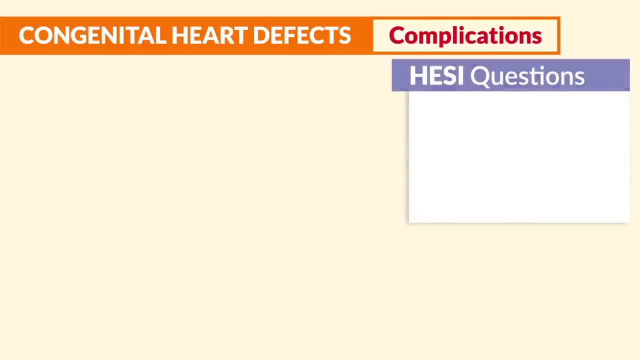 vessels and form a deadly blood clot, Specifically in those tiny blood vessels within the brain. Now this blood clot can cause a deadly stroke, a CVA, a cerebral vascular accident. So this is why we must report decrease the risk of blood clumping together and forming clots. So Hesse mentions polycythemia. 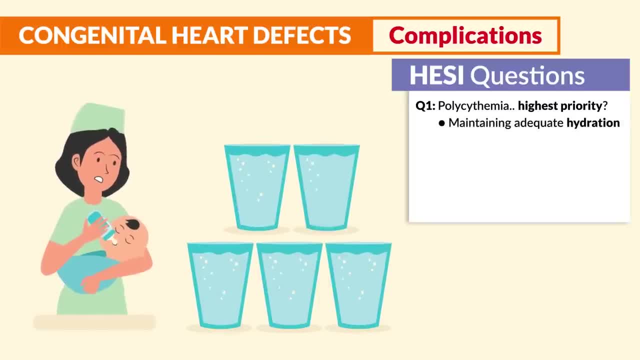 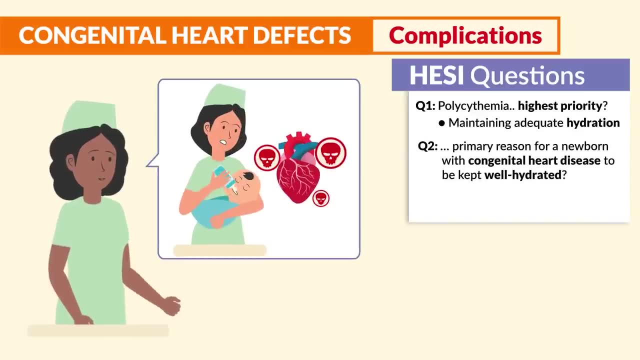 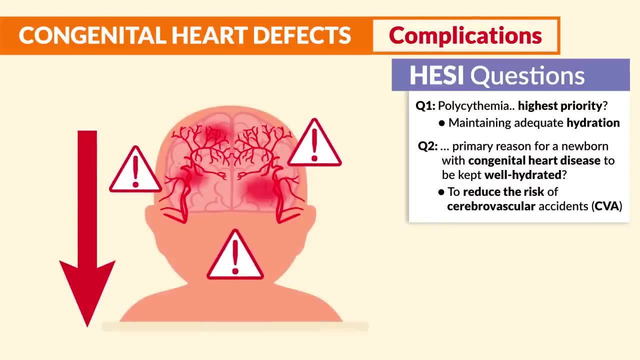 highest priority, maintaining adequate hydration. And question number two here: primary reason for a newborn with congenital heart disease to be kept well hydrated to reduce the risk of a cerebrovascular accident. the CVA Fancy words for a brain stroke. Now Kaplan mentions cyanotic. 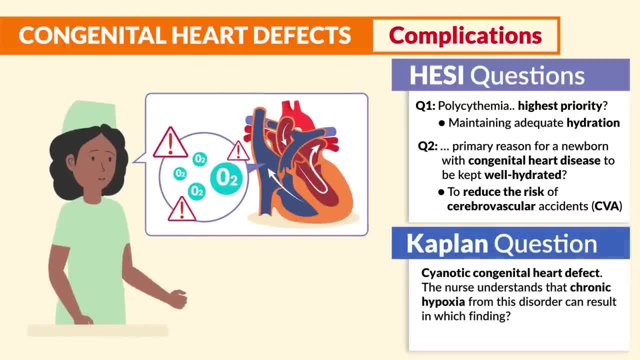 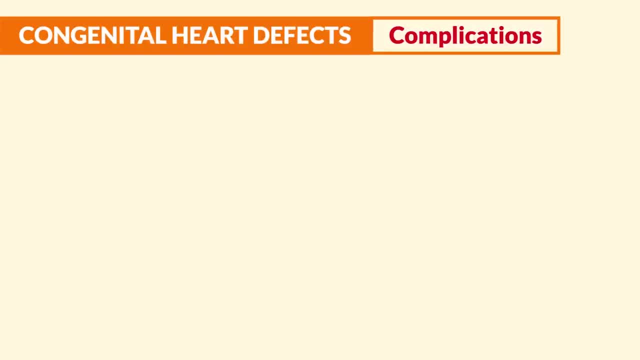 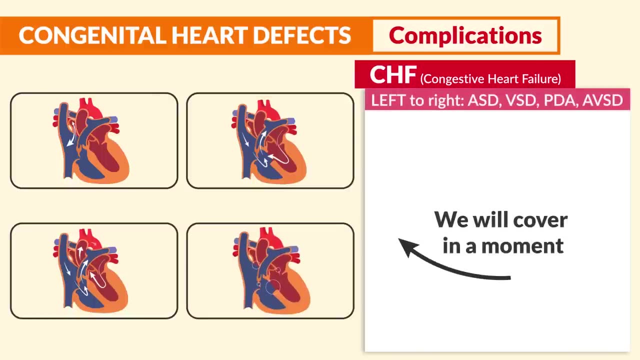 congenital heart defect. The nurse understands that chronic hypoxia from this disorder can result in which finding Polycythemia, Now switching gears to CHF, congestive heart failure. This is most common in left to right heart defects with ASD, VSD, PDA as well. 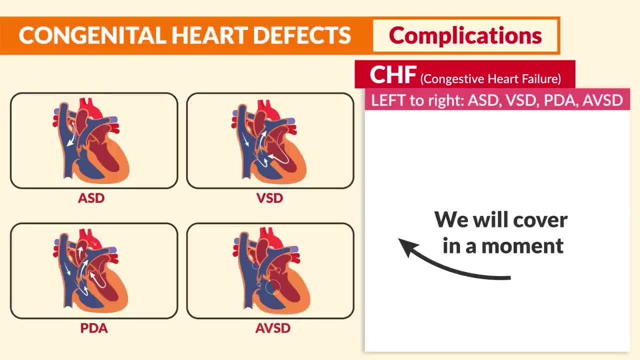 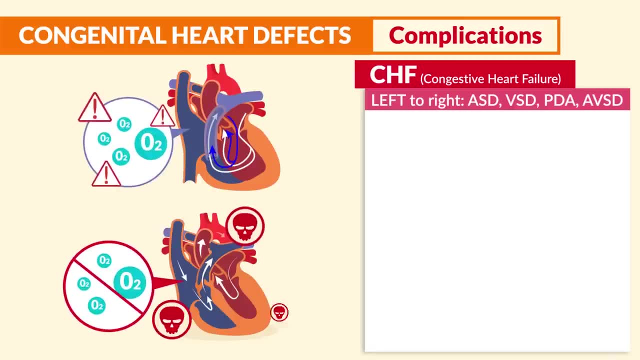 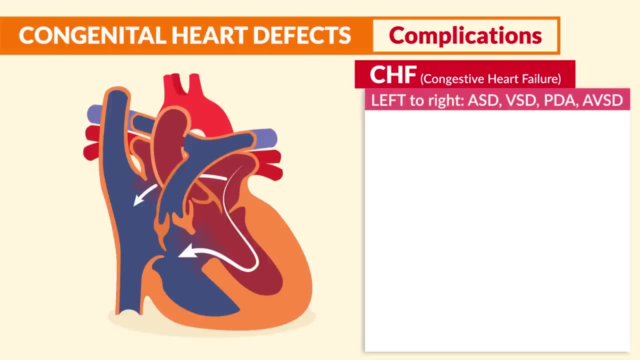 A-V-S-D And P-I-M-P. I'm just kidding. Okay, these are far less deadly than the right to left problems, as hypoxia is not a primary problem here. So these defects are from holes in the heart septum that push blood from the left side of the heart to the right side into the lungs.